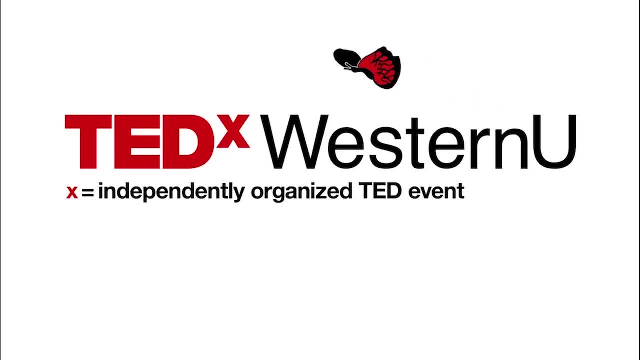 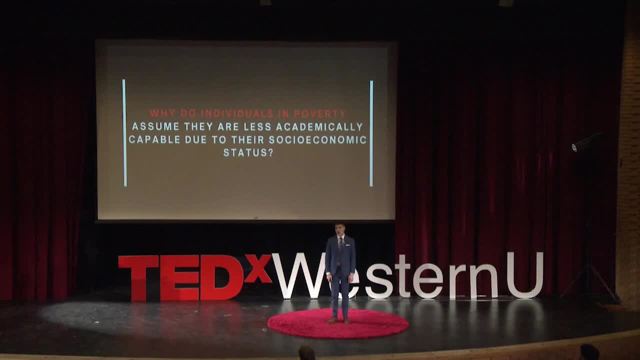 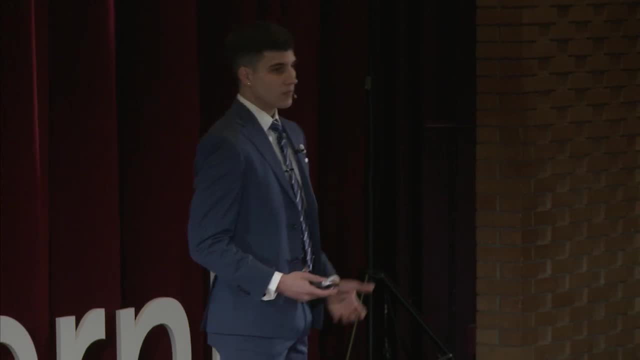 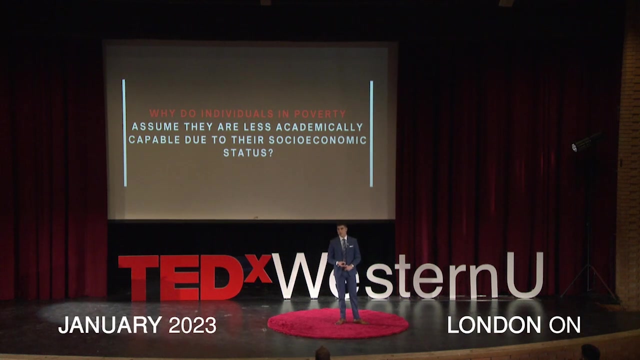 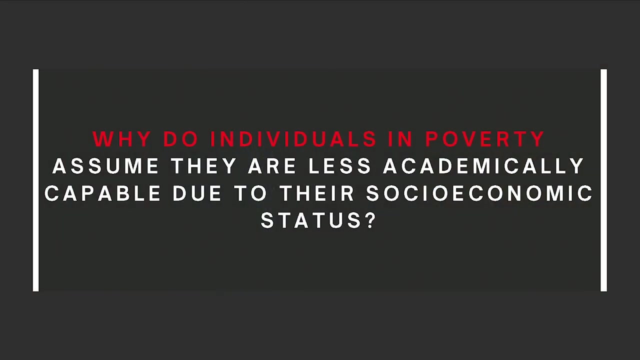 I thought I was different And I thought I was special. You see, I pondered these notions every time I entered an exam, worked on an assignment or sat down for an interview. But why is that? Why do individuals in poverty assume they are less academically capable? 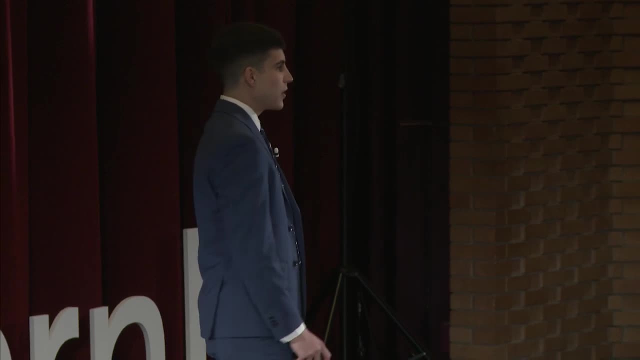 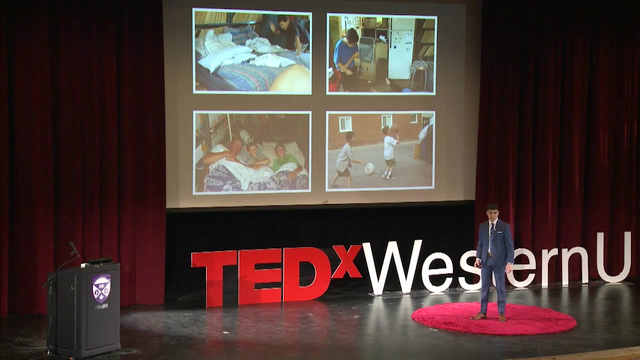 due to their socioeconomic status? The answer to this question is quite multifaceted, So let me illustrate my story to help shed some light on the issue. I was born and raised in Markham, Ontario, a city in the heart of the greater Toronto area where the average household has a net worth roughly $1.6 million. My family, however, was far from average. Growing up, my parents had a combined income of $40,000 Canadian dollars. Due to their minimal cash flow, I was raised in a 700-square-foot. 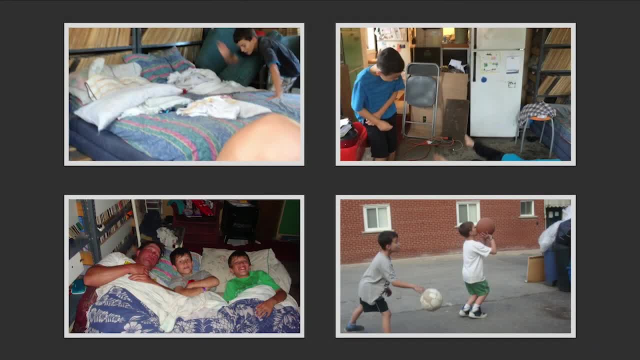 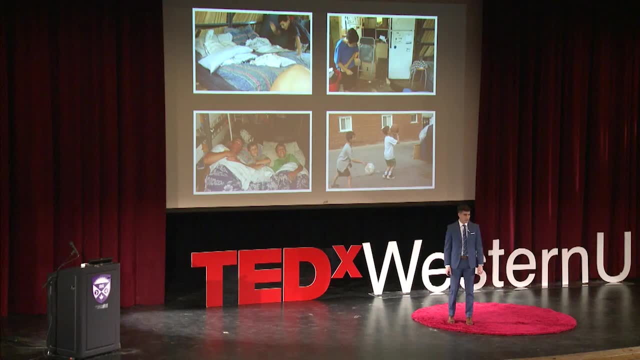 two-bedroom, one-bathroom apartment roughly the size of a three-car garage. Our family of six made the living space feel minuscule. As my brothers, Mateo Leo and I, grew older, we began to feel like giants standing in a miniature kingdom. 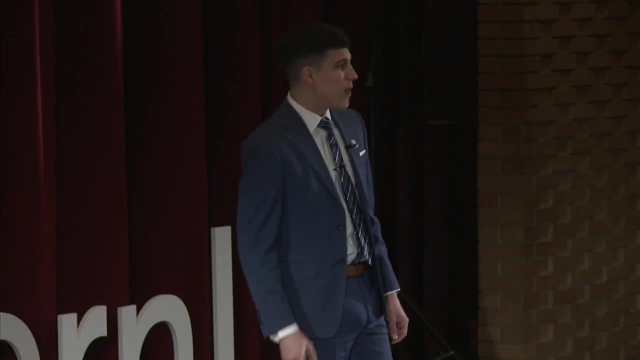 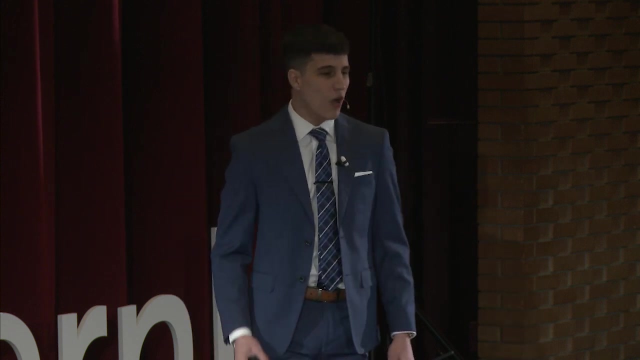 Every night, my mother would lay foam mattresses down on the ground to build a bed for us, which she would then disassemble the following morning to create the space we called our living room. On a nightly basis, my brothers and I would fight over who got to sleep singly on the 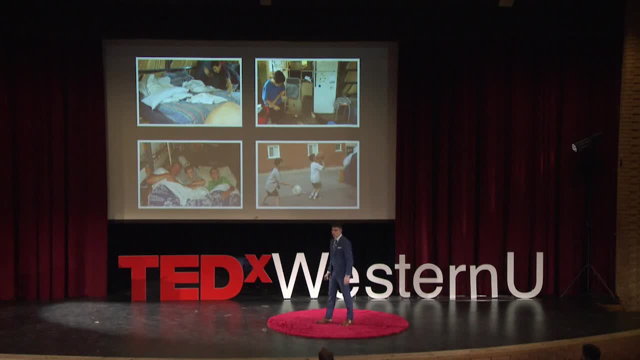 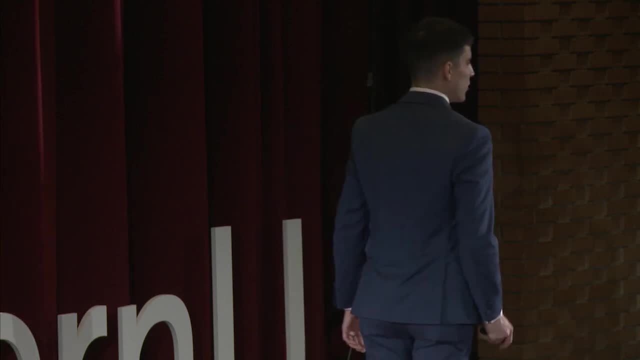 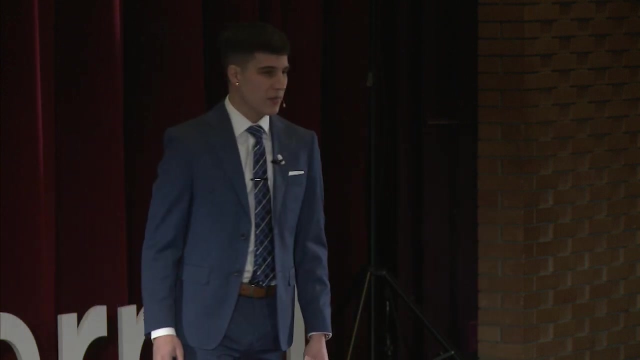 couch cushions and who had to share the makeshift bed. During the winters, we'd use space heaters to keep warm, and it would keep the apartment just warm enough that we only saw our breath in the very morning. I will never forget the time that I awoke to my parents screaming because the space 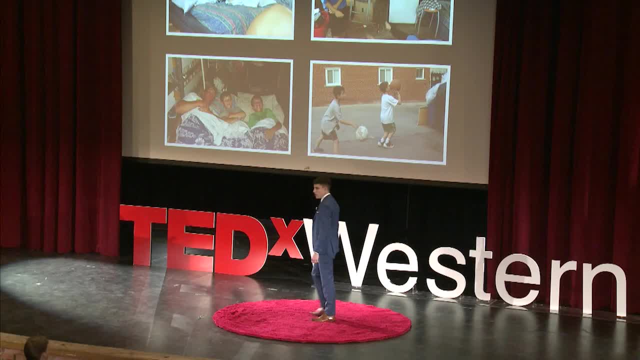 heater at the feet of my couch bed had caught fire. During our free time, my brothers and I would play basketball against the electrical poles in the shared driveway we called our backyard. Although I grew up in suboptimal living conditions, my life could have always. 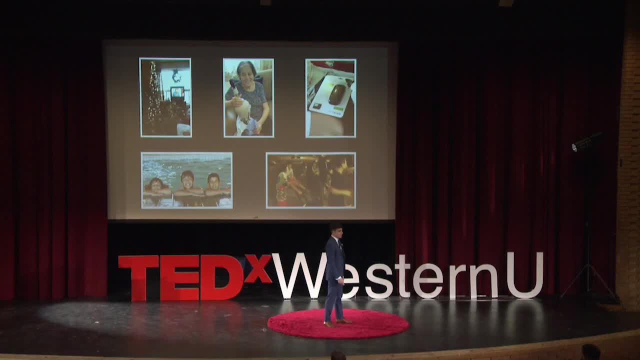 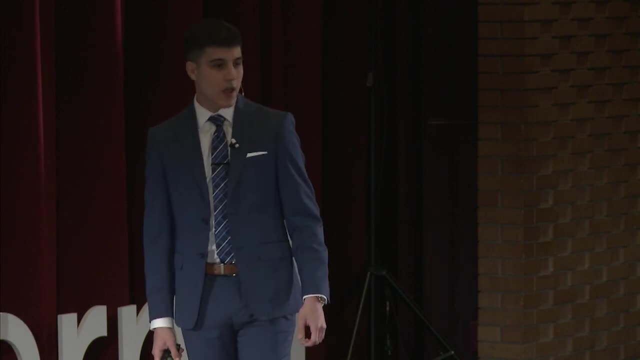 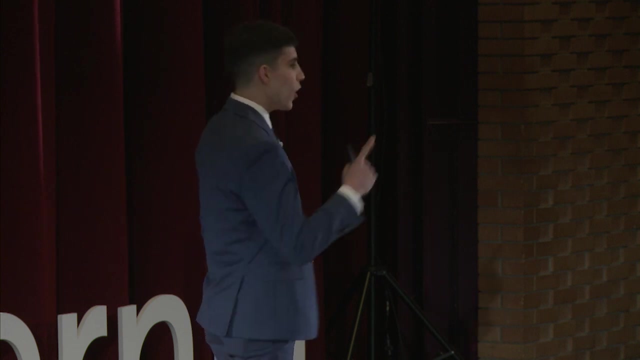 satisfied with the food we ate. When the holidays came round, my brothers and I would spend the weeks leading up stealing each other's things to give us more presents to open on Christmas Day. There was one time we even stole my grandma's side table lamp and she didn't even notice. 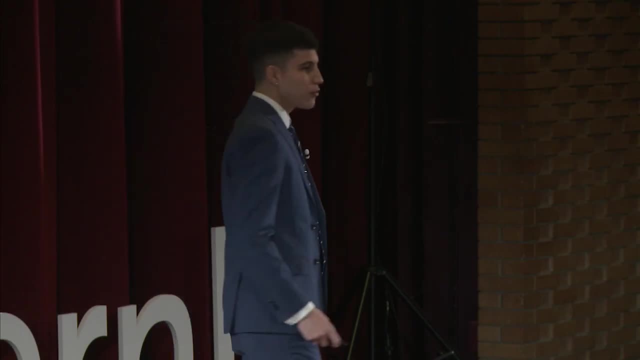 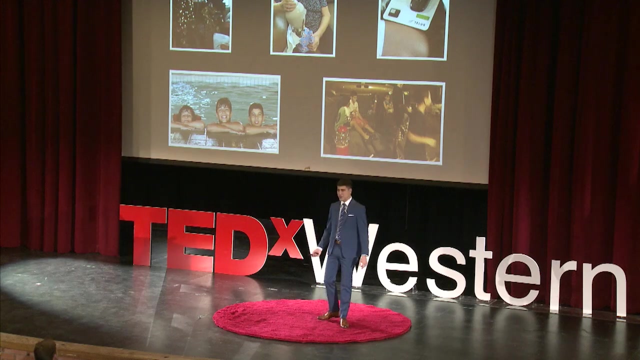 until the morning of. My parents tried your best to provide us with non-essential resources, and although I only got a prepaid flip phone that I top up each month with 25 calls and 250 texts, at least I had a phone. When it came to vacation time, I locked myself out. This is not what I had in mind. There was noơ. I needed something, but I didn't have. 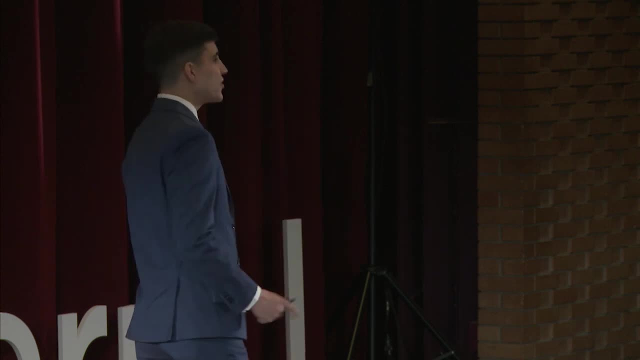 vacation time, we'd head over to Niagara Falls, where we'd share a $60 motel room and swim away in the pool we wish was in our own backyard. We even managed to have some get-togethers outside, where we'd carry our couch downstairs into the driveway and create a makeshift playroom As I grew older, I quickly began to realize that my life was not like others, And I worked very hard to hide this from my peers, And it was successful. Directly after becoming a teenager, I quickly secured my first part-time job, working 22 hours a week to completely remove the financial burden. 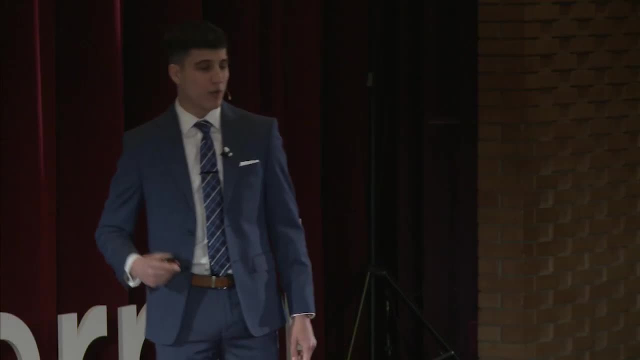 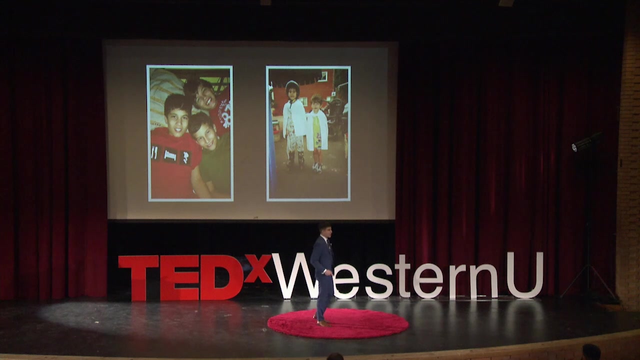 of myself from my parents. The stigma of poverty that I was running from, however, had substantial implications on my self-esteem, leading me to believe that I was not academically capable due to my socioeconomic status. During my public and high school years, my parents provided us with the 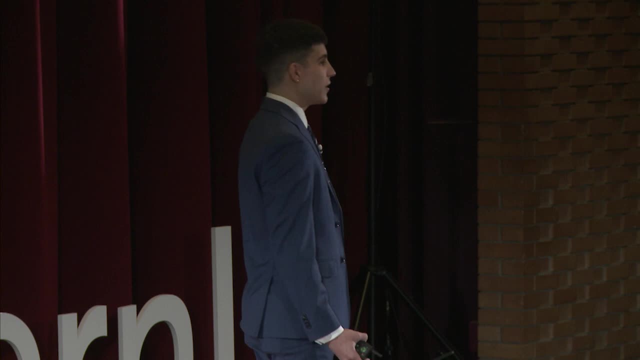 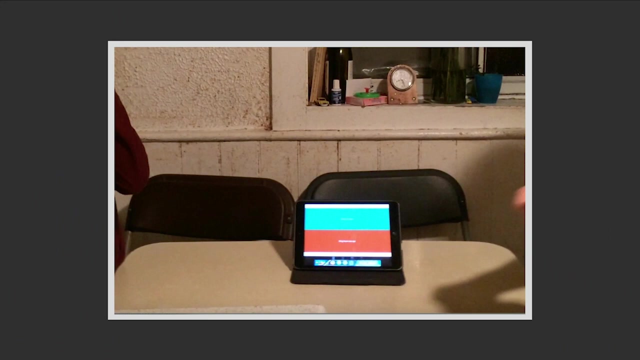 best resources they could afford and we utilized them to the best of our ability. During this time, my study space consisted of this old kitchen table with two pieces of paper under two of its legs to offset the slanted floor of the apartment. Alongside my brothers crying as my parents argued over money. 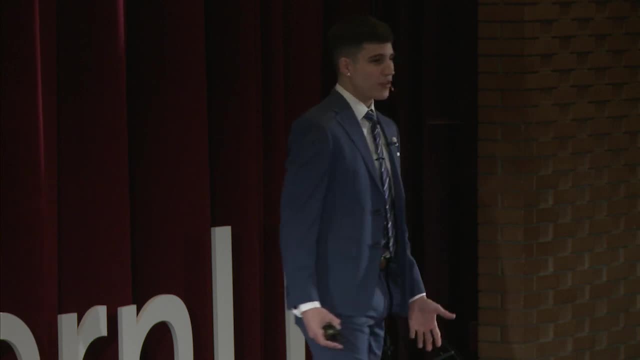 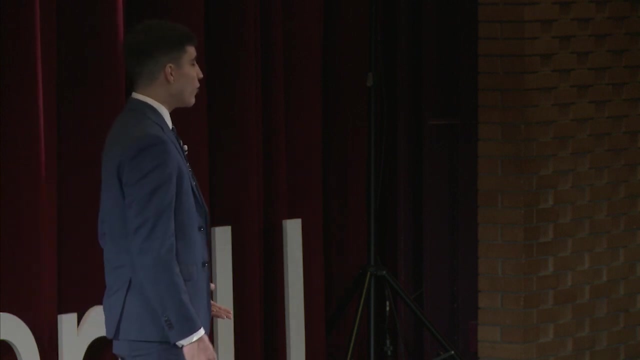 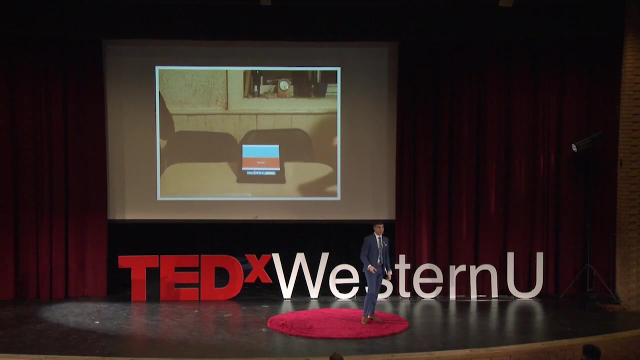 It was very difficult to study The loud noise, the lack of personal space And, because of this, my academic growth was negatively affected. The decrease in self-esteem coupled with the slowed academic growth resulted in my academic capability being negatively affected And because of this, 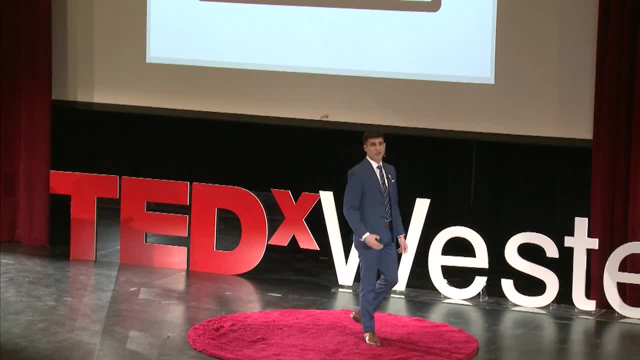